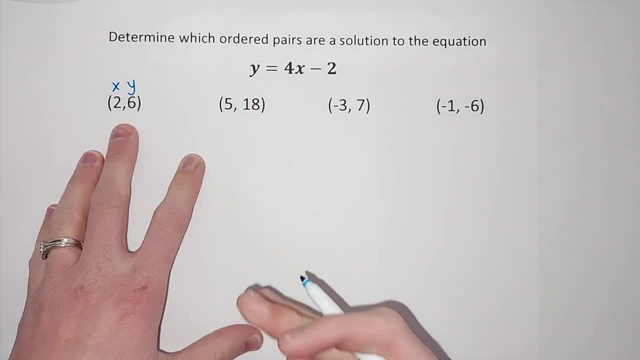 could be graphed as a line and we're wondering if these points are on that line. okay, So to do that, we're going to plug in our first number for x, our second number for y and see what happens. 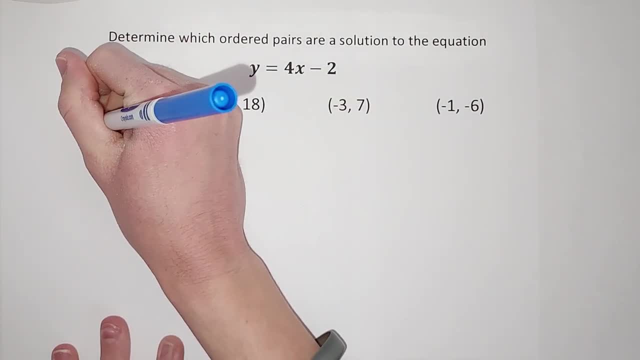 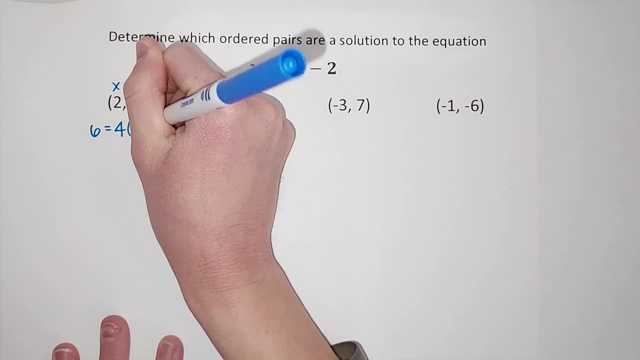 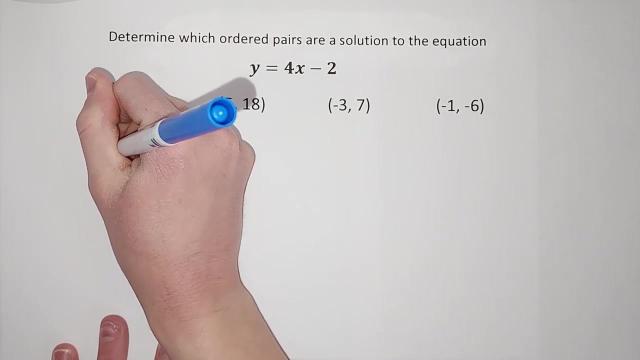 okay, So I've got y equals, so I'm going to write it as: 6 equals 4 times x, which is 2, minus 2, okay, Order of operations. I multiply first, so I'm going to do: 6 equals 4 times 2 gives me 8 minus 2, okay, 8 minus 2 gives me 6, so I end up. 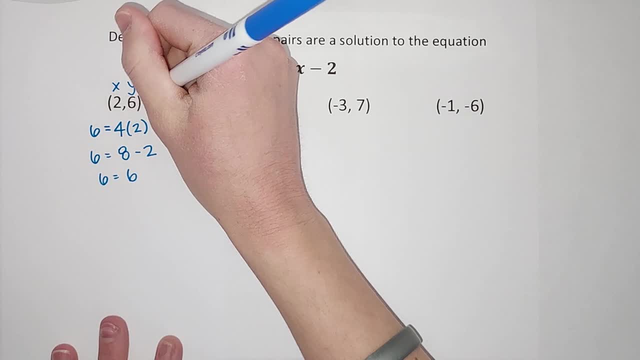 with 6 equals 6,, which is true. So, yes, this ordered pair is a solution. If we were to graph this line 2,, 6 would be on it. okay, All right, let's look at our second one. Again, my first. 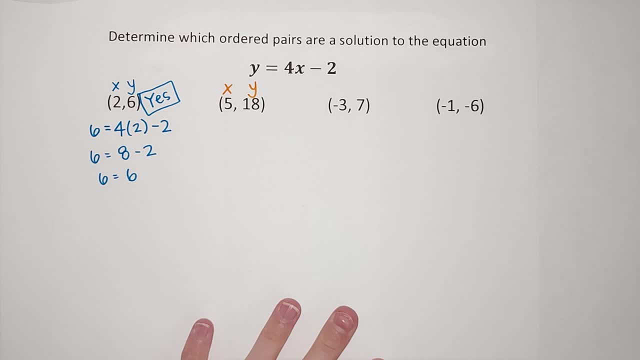 number is considered my x. my second number is considered my y. my second number is considered my y. okay, So I'm going to write this as: 18 equals 4 times x, which is 5, or we're seeing if. 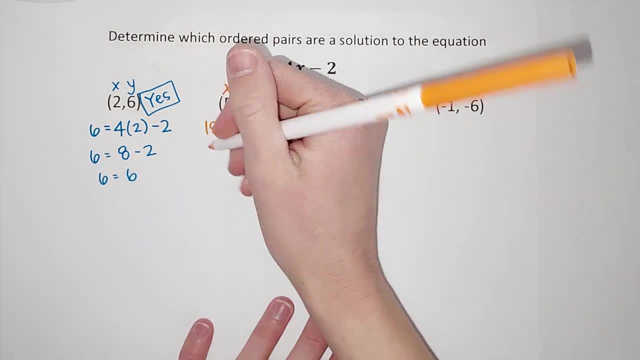 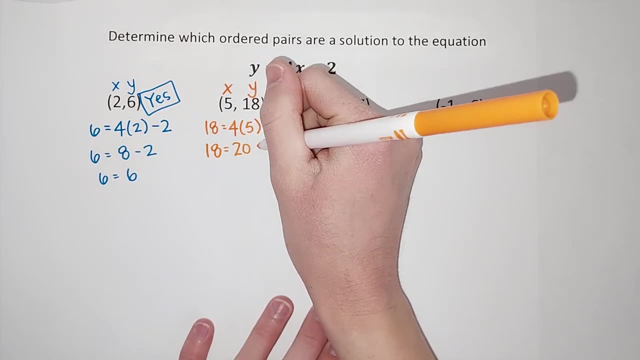 it can be 5, minus 2, okay, So I'm going to have 18 equals 4 times 5 gives me 20.. We still have the minus 2, okay. 20 minus 2 is 18, so I end up with 18 equals 18.. 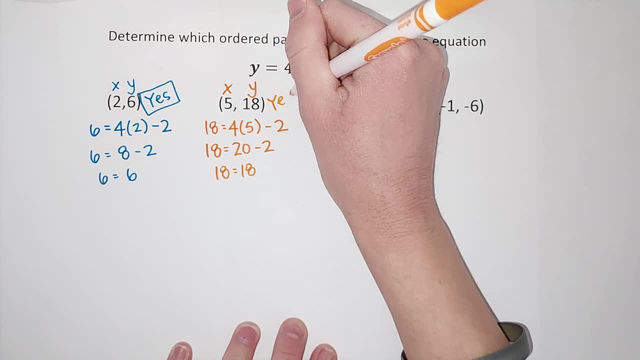 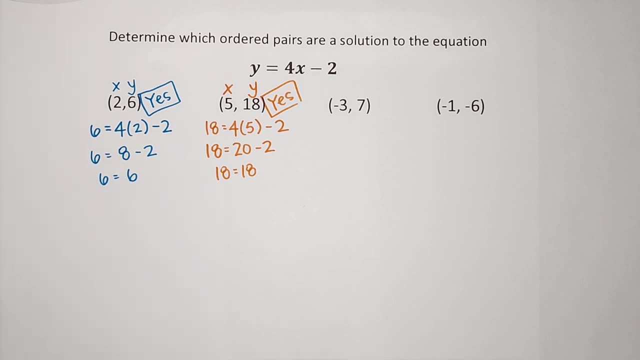 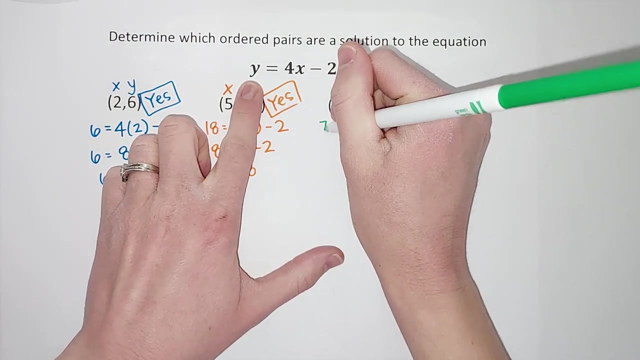 Which is true. So, yes, this one is also a solution. Okay now, oh, we've got one with a negative, but we can handle it. First one is my x, second one is my y. okay, So y equals 7 equals. 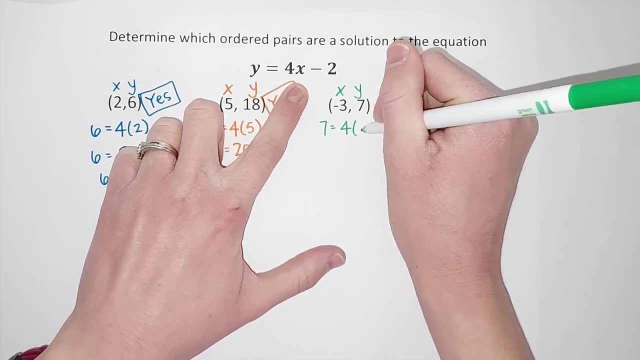 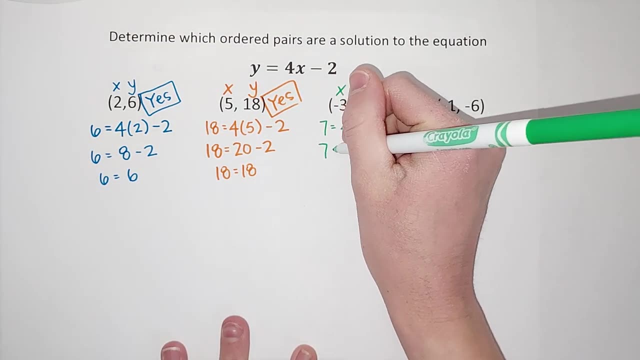 4 times x, which we are seeing. if it can be negative 3, minus 2,, okay, All right, I'm going to multiply first. so 7 equals 4 times negative, 3, positive times a negative gives me a negative 12 minus 2.. Oh, not looking. 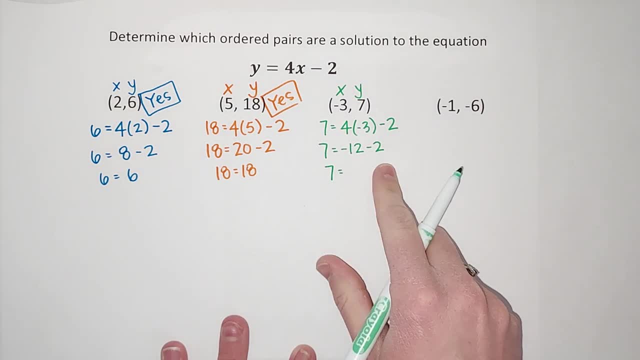 good, right, We're going to end up with: 7 equals negative 12 minus 2.. That's like I owe you $12, I borrow two more dollars, so now I owe you $14.. All right, 7 does not equal negative 14, right.